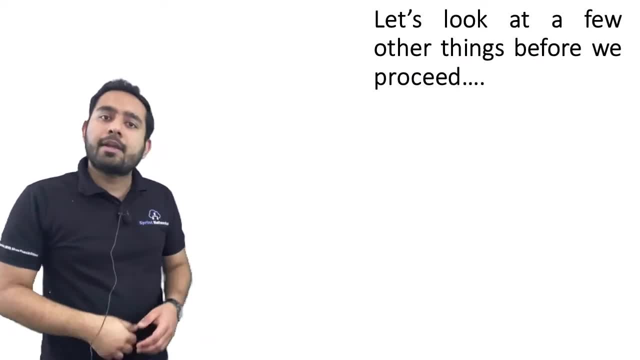 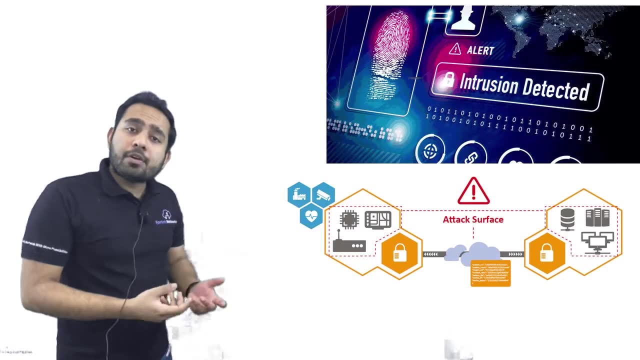 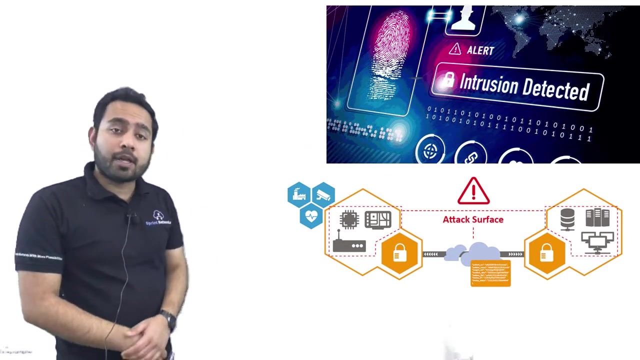 So, guys, before we go any deeper into this topic, let's try and do a little bit of background, as in trying to understand the vulnerabilities facing a typical network. So a breach or an intrusion is any unauthorized access or activity In a network or computer system. threat actors exploit diverse methods and vulnerabilities to access confidential resources, steal private data, alter data, destroy resources or block access to resources, with the goal of impairing productive business operations. 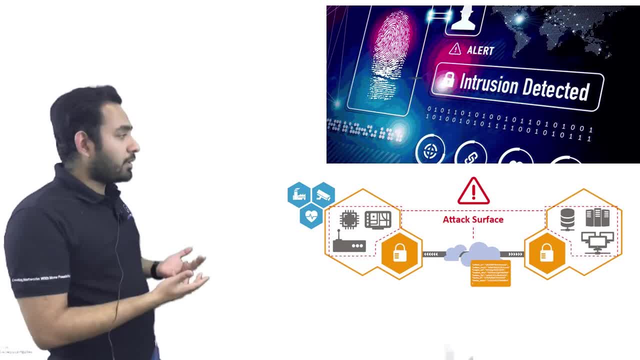 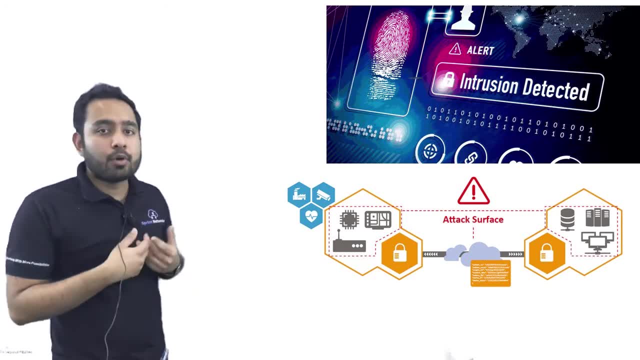 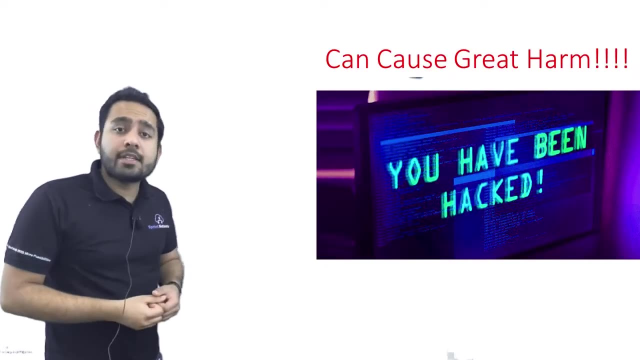 The attack surface is the area of your network and other digital operations potentially open to intrusion by unauthorized access. The more connected your network and resources are, the broader the attack surface is. So how do these systems detect or deal with threats? Well, these systems detect suspicious or unauthorized activities, such as: 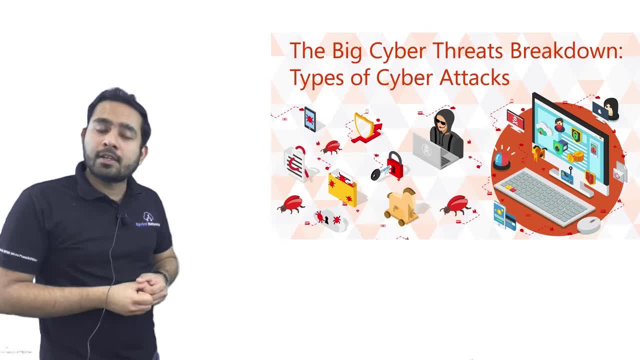 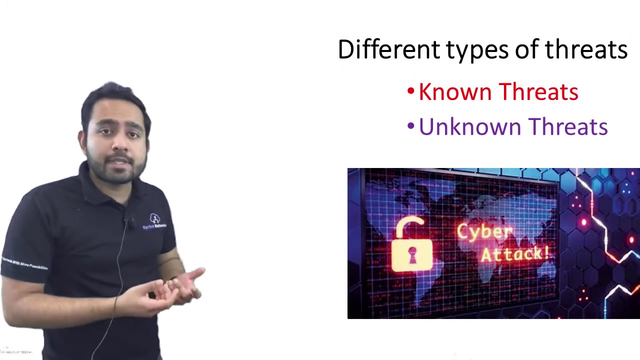 Phishing attacks, Virus infection and distribution, Malware and ransomware, Reinstallation and download, Denial of service or DOS Man in the middle, attacks, Zero-day attacks, SQL Injections, injection, while cyber attacks trend towards increasing sophistication over a period of time. well, there are two different types of threats, so known threats are typically detected by matching. 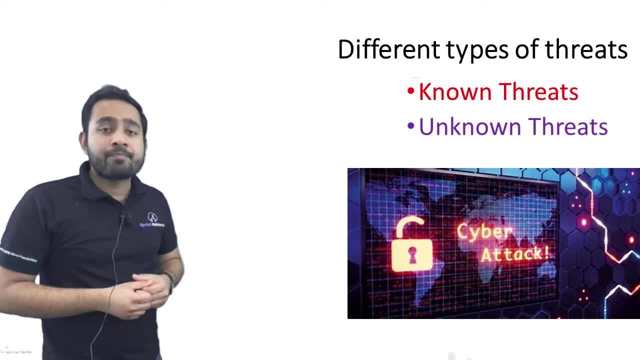 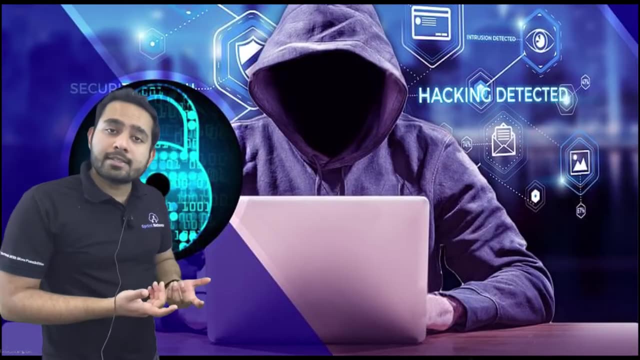 traffic patterns against signature patterns. frequently updated databases contain vast rows of signatures characterizing existing threats, so these systems continuously look for matches against known signatures, whereas unknown threats are malicious patterns never seen before, sometimes evasive variations of known threats and are significantly more difficult to detect. so these systems use behavioral analysis to pinpoint potentially. 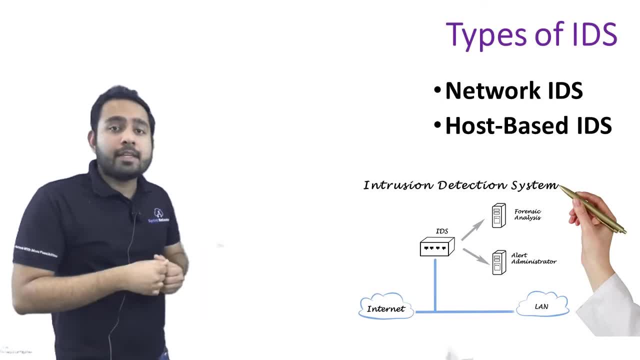 harmful traffic patterns. so what are the different types of ids or intrusion detection systems? well, intrusion detection systems generally come in two flavors. well, what are they? let's have a look. so network intrusion detection systems, or nids. this system is part of the network infrastructure and monitors packets as they flow through the network. nids usually co-decides with 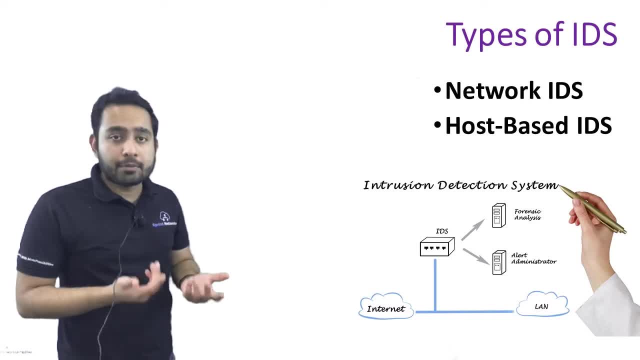 devices that have span, tap or mirroring capability, such as switches. the other one is host-based intrusion detection system, or hids. this software resides on client computer or server devices and monitors events and files on the device. well, let's look at the different types of intrusion. 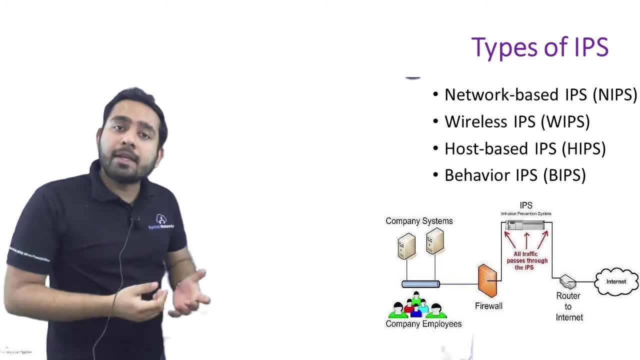 protection systems, or ips. well, there are multiple types of intrusion protection systems. the first one is network-based intrusion prevention system, or nips. so this system is deployed in line in the network infrastructure and examines all traffic in the entire network. the second one is wireless intrusion prevention system, or wips. 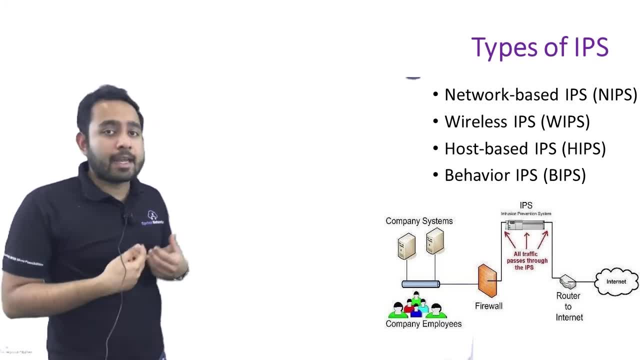 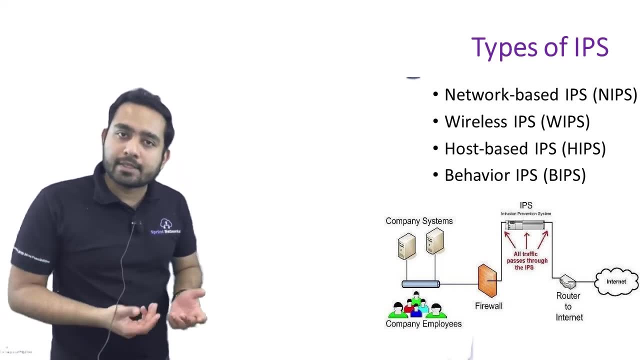 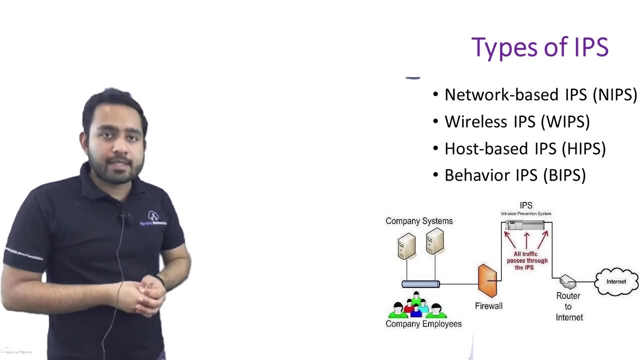 this system is part of the wireless network infrastructure and examines all wireless traffic. the third one is host-based intrusion prevention system, or hips, so this software resides on the client computer or server devices and monitors events and files on the device. and finally we've got behavior ips. so this system is 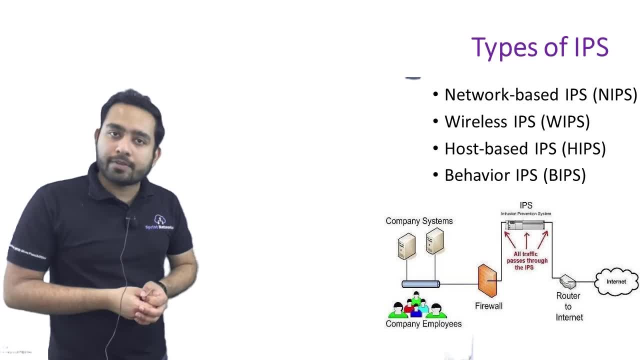 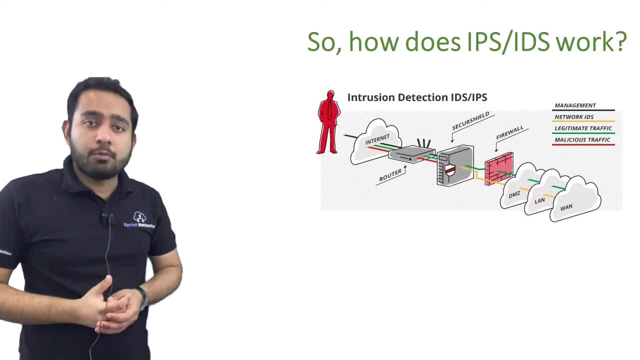 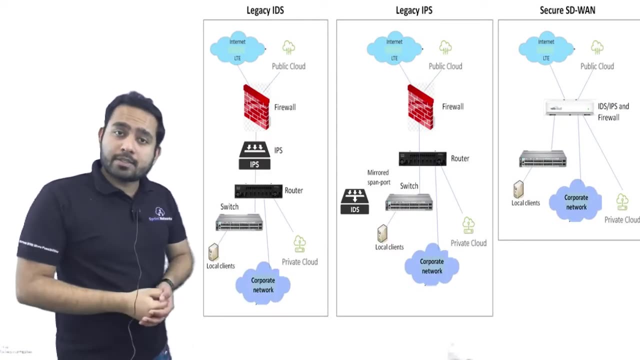 part of the network infrastructure and examines all traffic for unusual patterns and behavior in the entire network. So how do IPS and IDS work in Sprint Networks managed Versa Secure SD-WAN. Well, let me show you how. So here's how it works: Versa. 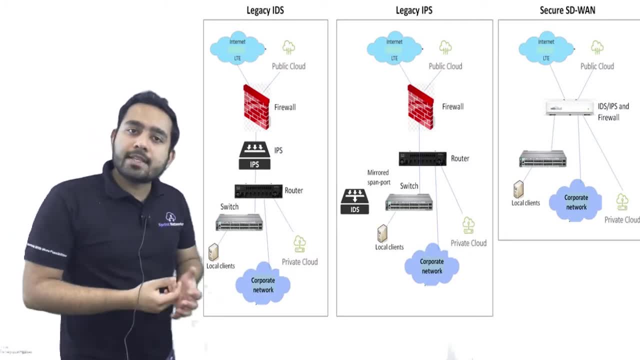 Secure Cloud IP architecture offers a unique, secure SD-WAN solution in an integrated single stack hardware agnostic software only offering that scales to the needs of any network. The integration of security into the very fabric of the solution simplifies your network architecture, reduces the number. 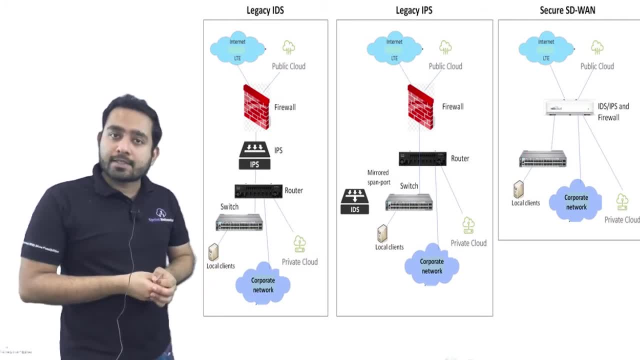 of devices to manage and limits the attack surface. So the Versa Secure SD-WAN single pass parallel processing architecture ensures the highest IDS IPS inspection performance and obviates the need for dedicated single-purpose intrusion inspection devices. Ground-up integration of security within the Versa. stack ensures full IP monitoring and performance, and also instructors can see how the security is integrated into the network. So The Versa Secure SD-WAN single-pass parallel processing architecture ensures the highest IDS IPS inspection performance and obviates the need for dedicated single-purpose intrusion inspection devices.